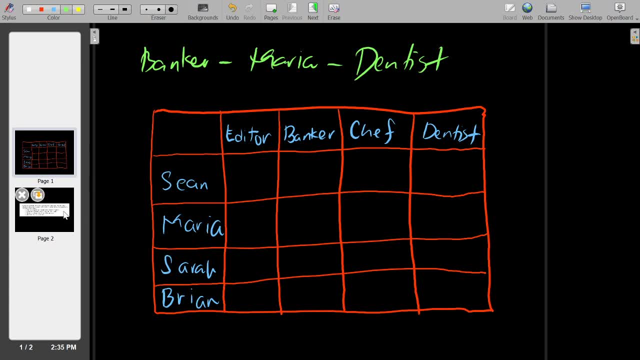 And then the second clue says that: Okay, going back to the first clue, Obviously from the first clue Maria is not the banker, So probably we can mark here some X. Okay, so Maria is not the banker. And then also Maria is not the dentist. 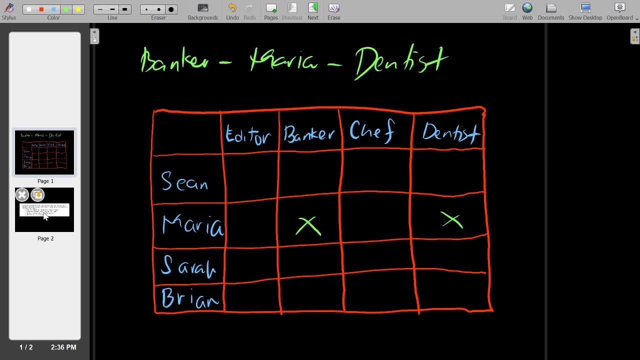 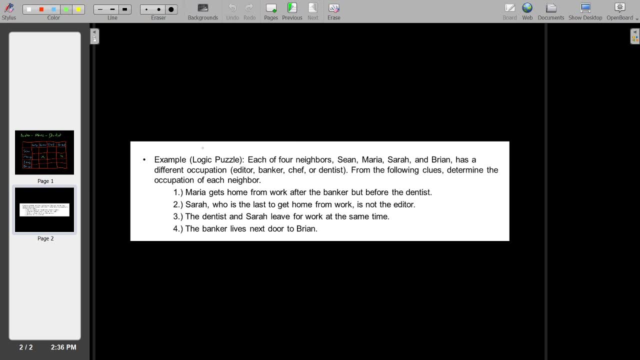 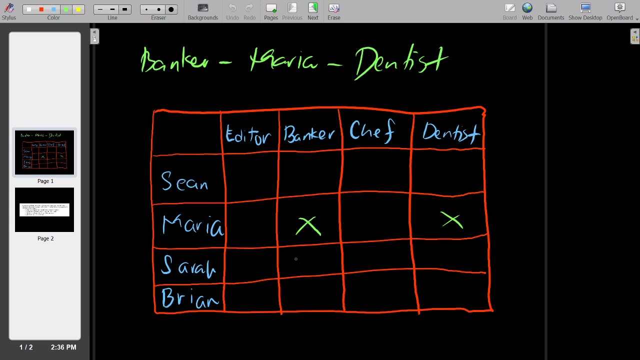 So that's coming from the first clue. Okay, let's go to our second clue. Sarah, who is the last to get home from work, is not the editor. Okay, so obviously Sarah. So probably we can also mark X. 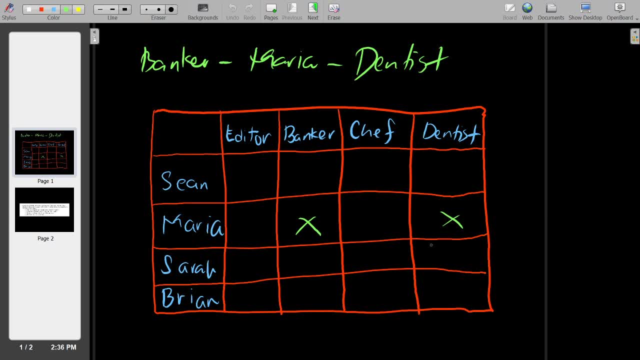 Sarah, who is the last to get home from work, is not the editor, So Sarah is not the editor. Okay, so from the second clue it says that Sarah is the last to get home from work, So probably we can write here: Sarah. 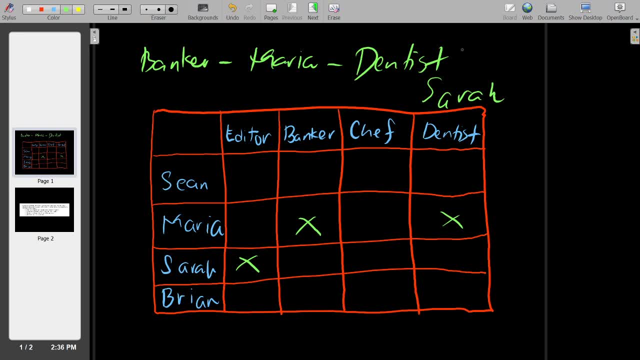 So probably Sarah can be a dentist. Okay, so Sarah is the last to get home from work. So still from the second clue: obviously Sarah is not the banker, Because Sarah is the last to get home from work And the banker comes home before Maria. 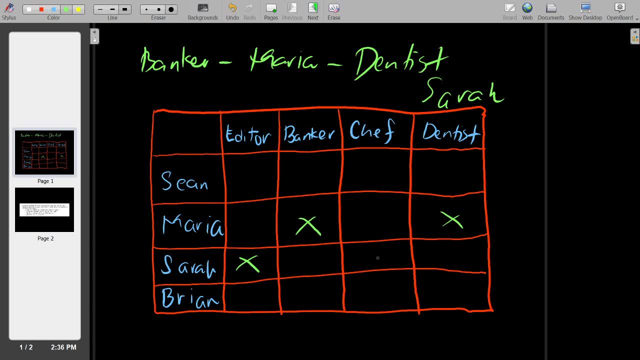 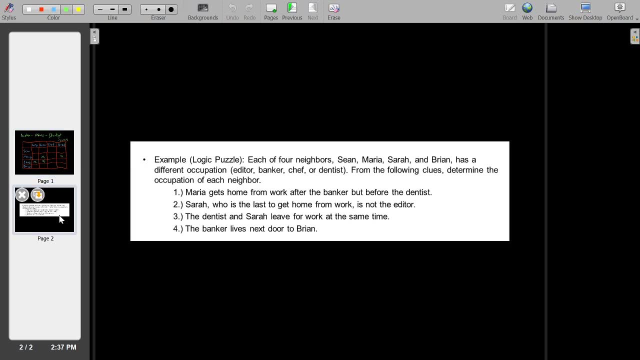 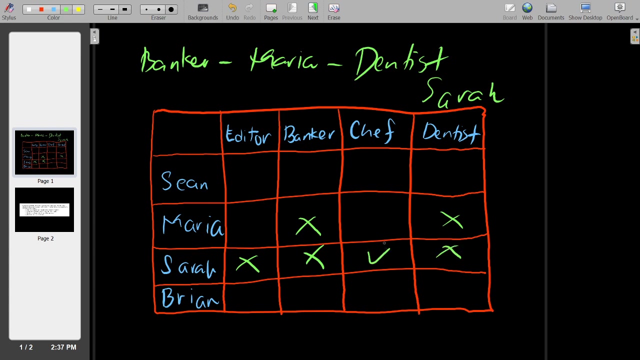 So we can mark an X here. Sarah is not a banker. Okay, so let's go to our third clue. The dentist and Sarah leave for work at the same time, So Sarah obviously is not the dentist, So therefore Sarah is the chef. 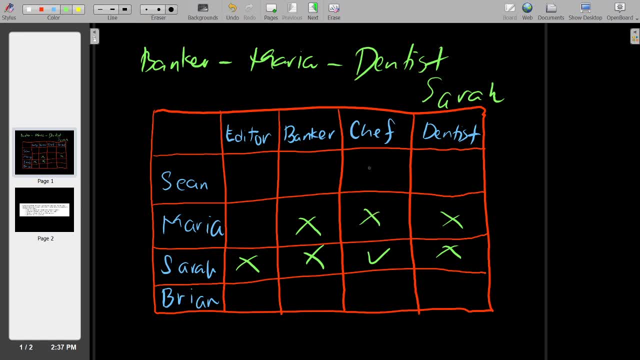 If Sarah is the chef, Maria is not the chef, Sean is not the chef And Brian also is not the chef. Okay, let's go to our last clue: The banker leaves next door to Brian And Brian is not the banker. 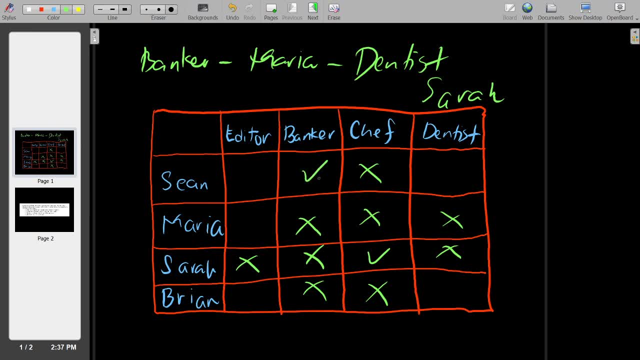 So if Brian is not the banker, Sarah is not the banker, Maria is not the banker, So Sean is the banker. So probably we can mark here as X And here Sean is not the dentist, Maria is not the dentist, And so on. 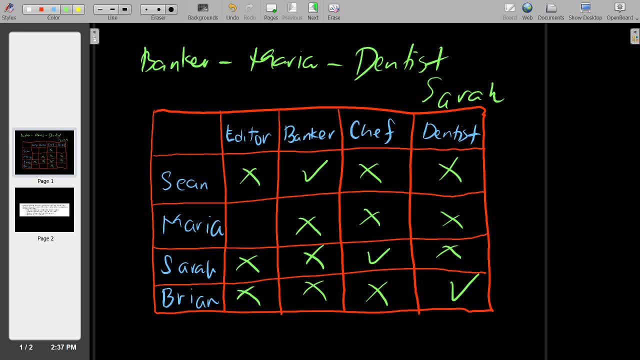 So Brian is the dentist? Okay, Brian is not the editor, So Maria is the editor. So, therefore, Sean is the banker, Maria is the editor, Sarah is the chef And Brian is the dentist.